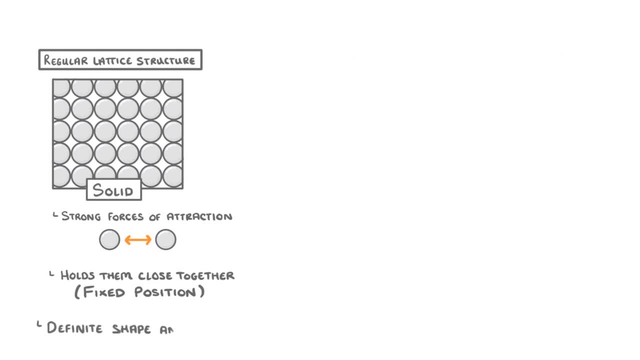 particles are fixed, the overall substance keeps a definite shape and volume, so can't flow like a liquid. The particles can vibrate in their position though, so you can imagine them constantly jostling against each other. Now, if we heat up a solid, its particles gain. 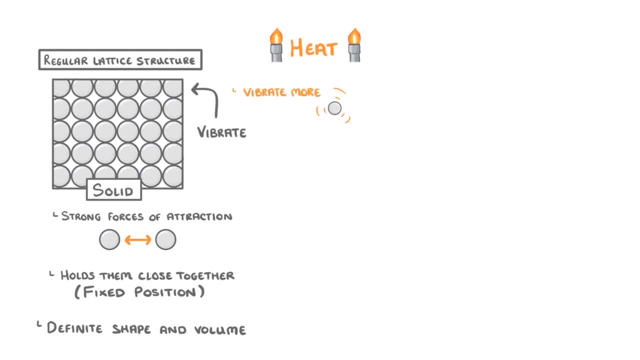 more energy and start to vibrate even more, which weakens the forces between them, And at a certain temperature, which we call the melting point, the particles have enough energy to break free of their bonds and the solid melts into a liquid. 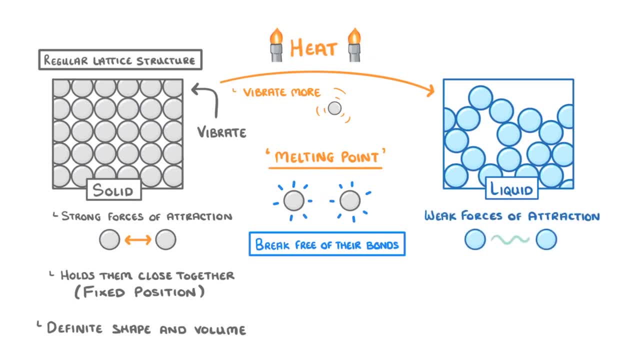 In liquids there are only weak forces of attraction between the particles, so they're free to move around and are arranged pretty randomly. However, the weak forces of attraction do mean that the particles tend to stick together and are fairly compact. This means that liquids have a definite volume, even though their overall shape can change. 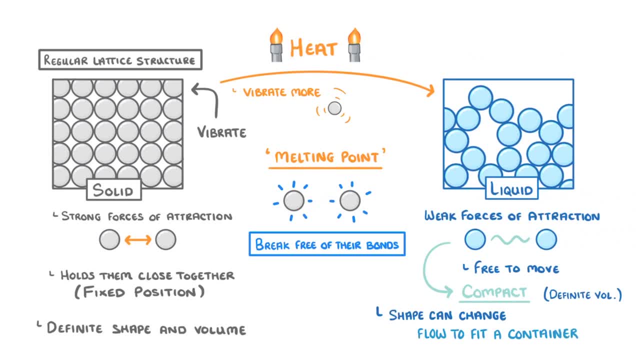 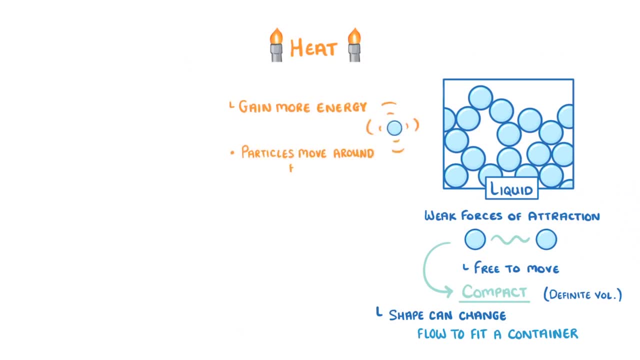 and so flow to fit a container. If we then heat up our liquid, the particles will gain more energy, and this will make the particles move around faster, which weakens the forces holding the particles together. Then, once we reach the boiling point, the particles will have enough energy to break. 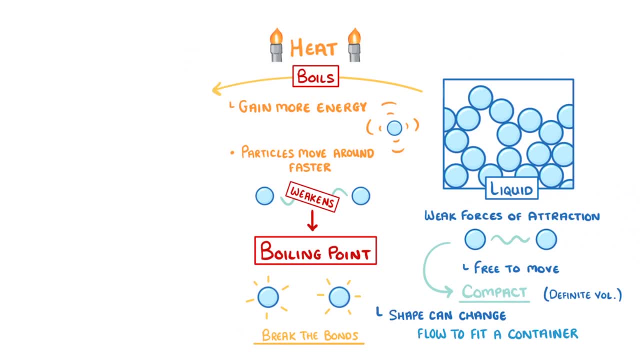 the bonds altogether, and so the liquid boils or evaporates. This means that the liquid will have enough energy to break the bonds altogether, and so the liquid boils or evaporates In gases. the force of attraction between the different particles is very weak, so they're. 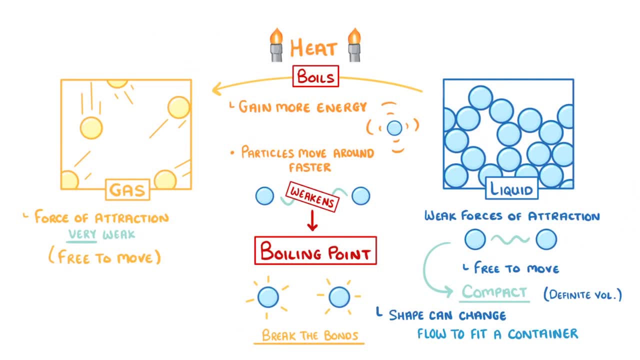 basically free to move around by themselves. This means that gases don't keep a definite shape or volume and instead will always fill a container as they spread out as much as possible. We normally say that gases are constantly moving with a random motion, and this can. 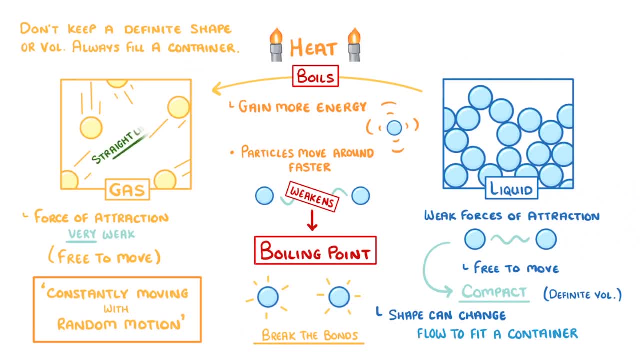 be a bit confusing, Because gas particles actually move in straight lines. They don't randomly swerve. What we actually mean by random motion is that particles can travel in any direction and they'll end up being deflected by solid walls or other gas particles randomly. 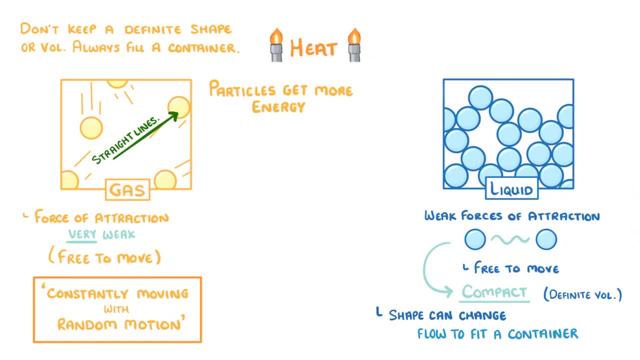 When we heat up a gas and the particles all get more energy and so travel faster, the gas will either expand if the container it's in is expandable like a balloon, or if the container is fixed. then the pressure will just increase.